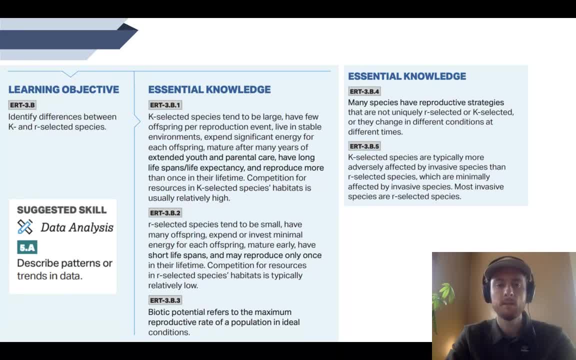 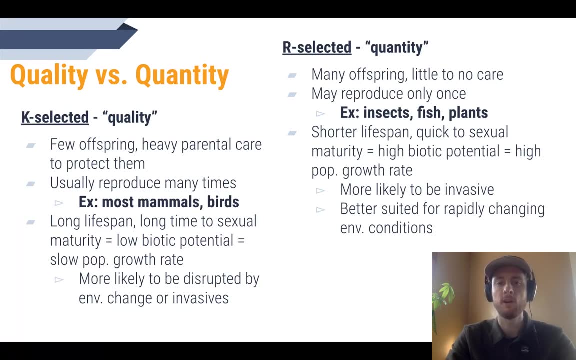 negatively impacted by invasive species. And then the science skill that we'll be practicing at the end of the lesson today is to be describing the patterns or trends in data. So, as I mentioned in the beginning, we have the reproductive strategies here- R and K-selected- and they sort of represent 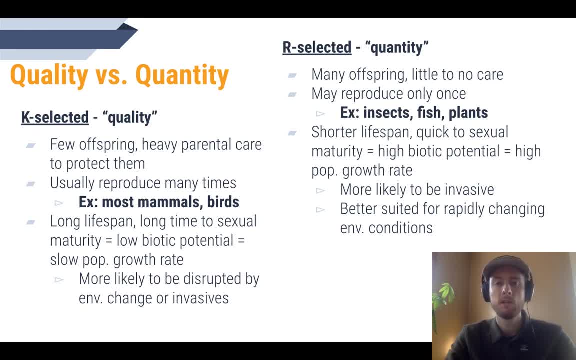 the quantity versus quality approach, And so, before we talk about the characteristics, we need to review that these are both reproductive strategies or approaches that different species take to passing on their genes. So all species pass on their genes to offspring. It's basically the. 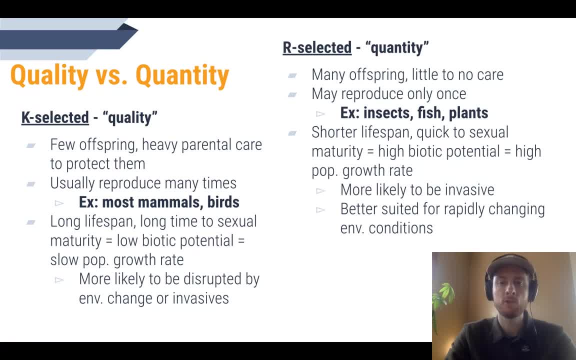 driving force behind all of life, And these are just two different approaches to accomplish that goal. They both work and they're both suited to the organisms that use them. And again we want to think of them as strategies and focusing on either quality or quantity. So K-selected species here. 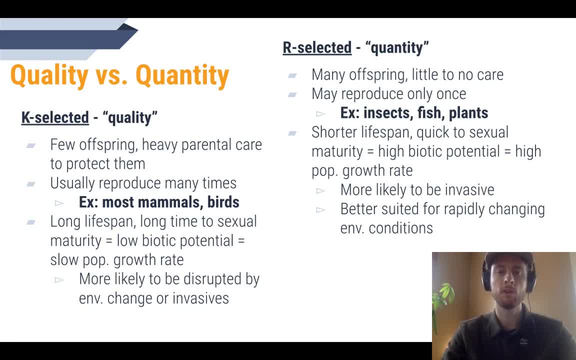 take the quality approach. They're typically larger, longer-lived animals, like large mammals, and they only have a few offspring at a time, but they take really good care of them. So because they live longer, they take longer to reach sexual maturity, but they also usually have the 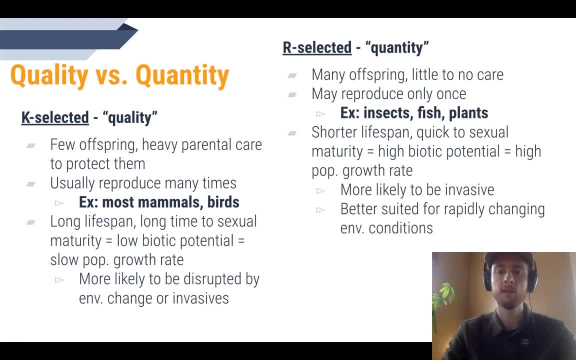 opportunity to reproduce many times over time. So that's one of the things that we're going to be looking at here. So we're going to look at the population population. So we're going to look at the population population over their lifespan. Since they only have a few organisms or a few offspring at a time, they invest. 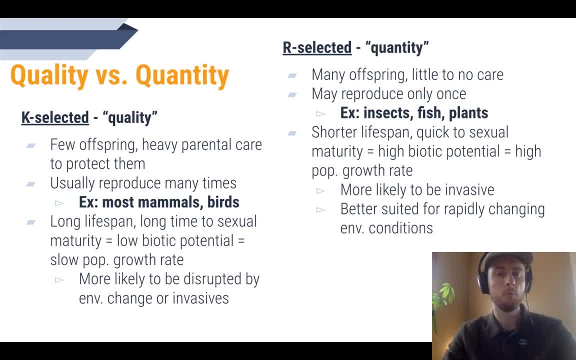 a lot of energy in them, They get them food, they keep them warm, and they might even fight off predators. Because of this, though, they have a lower biotic potential or maximum reproductive rate, which means they're going to exhibit slower population growth, Because it takes a long time. 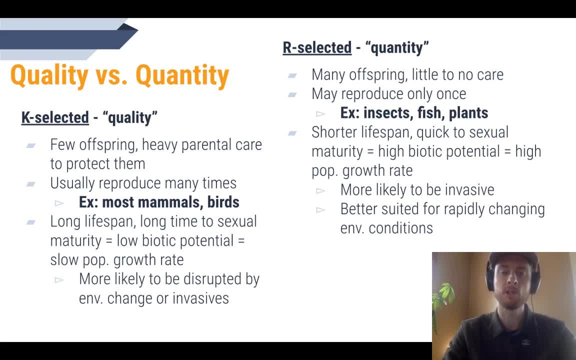 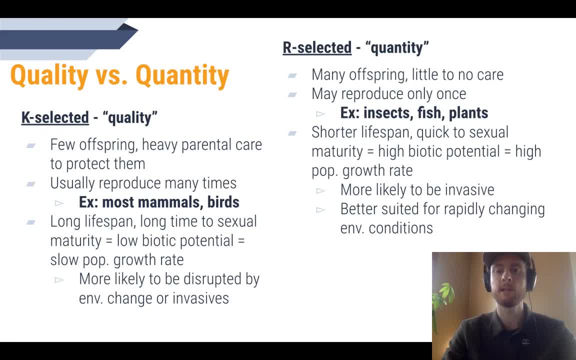 because their populations just take so long to recover back to that initial size. Our selected species, on the other hand, are going to take the quantity approach, So they're generally smaller, shorter-lived organisms like insects, fish and plants, And they often don't. 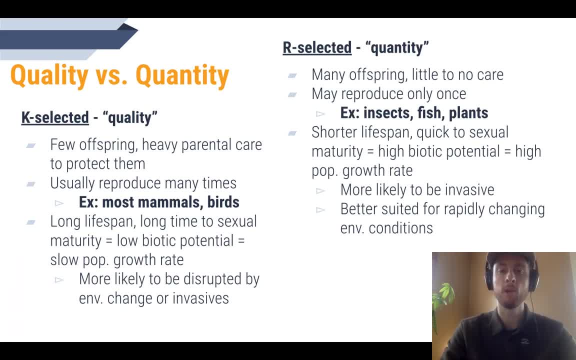 live enough to reproduce numerous times, So they really got to make that one-shot count, Because they don't live long, they've reached sexual maturity very quickly And they produce many offspring at one time. They invest their 50,000, don't dip, yeah. All of that trouble and dilation into food likeわか, without sample materials, and transport a energy in the production of this large number of offspring, but then they invest little to no energy in caring for them. So often there's no parental care at all, Since they don't care. 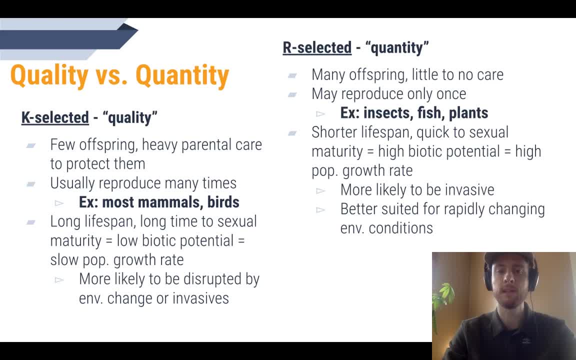 for them. they need to have a lot of offspring in order to ensure that at least some of them survive, So they have a very high biotic potential, or maximum reproductive rate. However, this reproductive rate can also make them more likely to become invasive species. 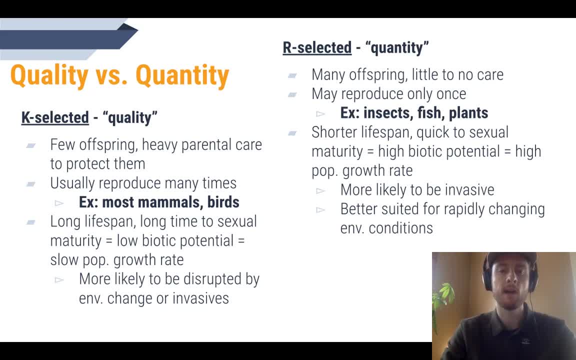 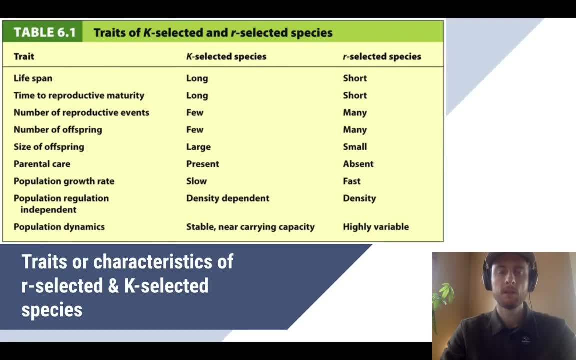 because their populations grow so rapidly they often out-compete slower K-selected species for resources like food or water. So here's a quick guide of the basic traits for both K-selected and R-selected species, And again, think of K-selected species as kind of taking their time. 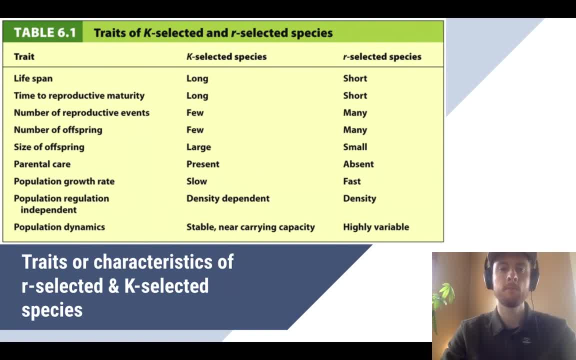 Slow and steady wins the race. They live a long time, so it takes them a long time to reach sexual maturity, And this also means that they have to protect and care for their offspring for a while, as those offspring grow And because their populations grow slowly, though they're usually relatively stable. 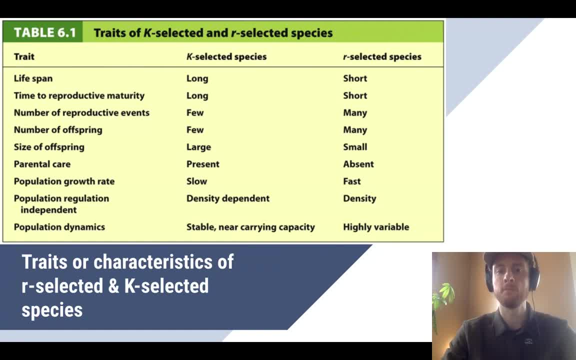 They exist near their caring capacity or their maximum population size. R-selected species are basically the opposite: They live short lifespans, they reach sexual maturity very quickly and they reproduce many offspring. They also invest their energy more in the production of offspring. 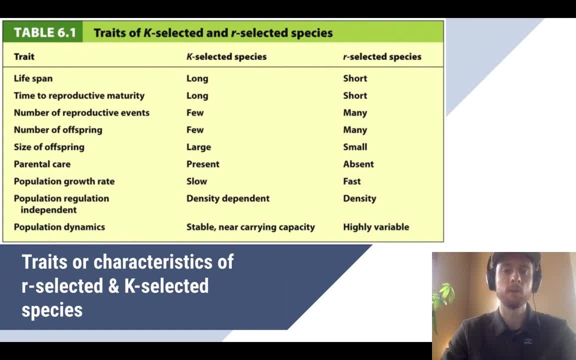 rather than caring for them. So it takes a lot of energy for a mother spider or a motheranimal- fish- to produce thousands and thousands of eggs, and then they don't invest that energy in caring for them. So this leads to them having very fast population growths but very variable population. 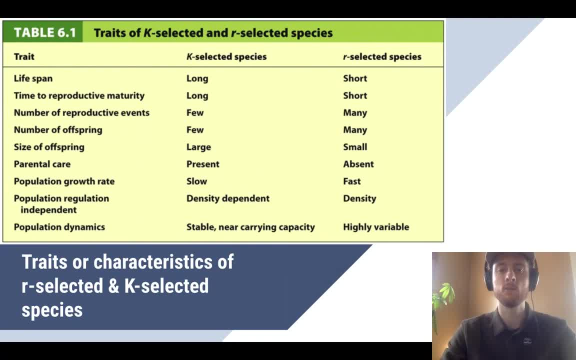 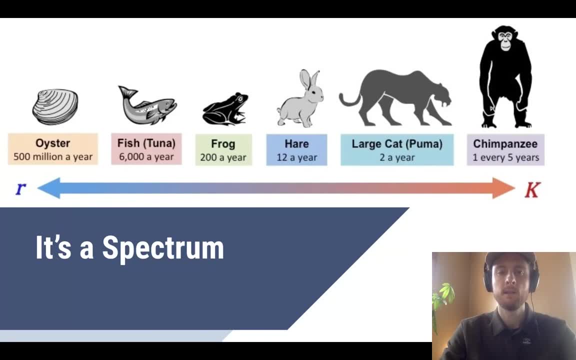 sizes, since they're subject to kind of dramatic increases or decreases. So it's important to remember that not every organism is perfectly K-selected or R-selected. We can see here two extreme examples of a highly K-selected organism: the chimp, or a highly R-selected oyster. 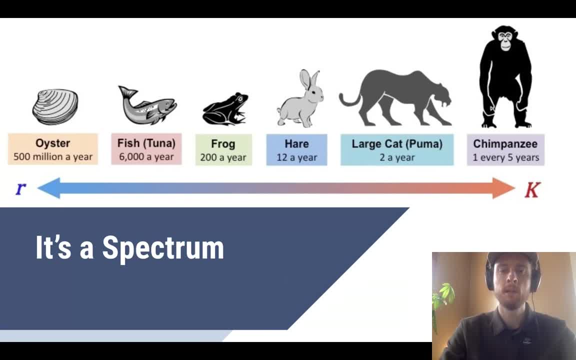 But you'll notice, here there's many species that are somewhere in the middle, like the frog and the hare. So the frog and the hare are going to produce a fair number of offspring compared to the chimp, but they're also going to show some parental care compared to the. 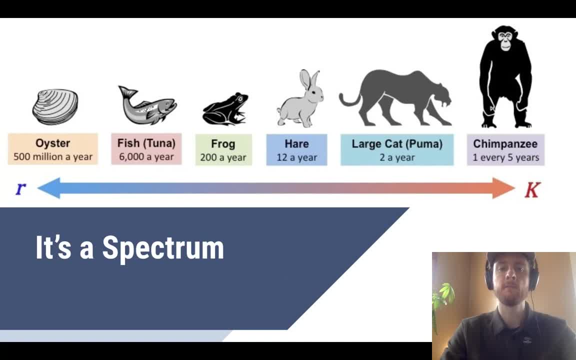 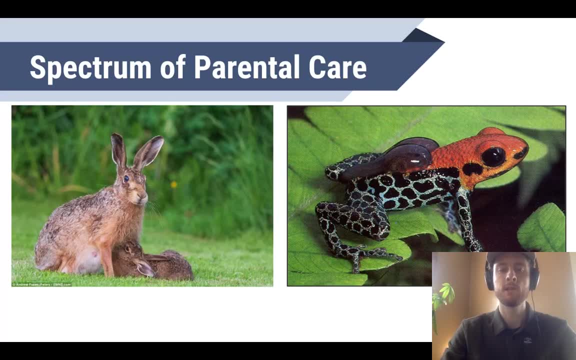 oyster. So not every single organism fits perfectly into R-selected or K-selected. It is kind of a spectrum. So here we have the mother hare who is going to provide quite a bit of care to her offspring. They're going to be somewhere in the range of 10 to 12 at a time. 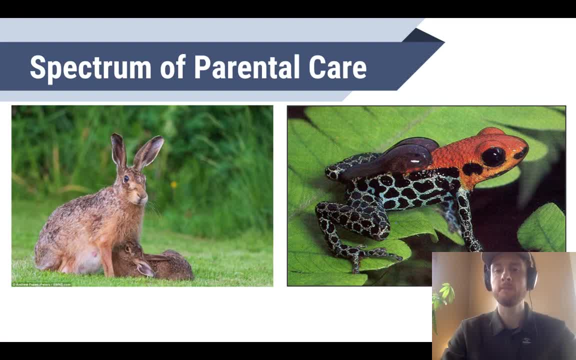 And frogs, even though they may have hundreds of offspring in a reproductive cycle. many frogs offer some parental care, such as this poison dart frog here that's going to carry tadpoles on her back. So again, it's a spectrum. These organisms aren't going to exhibit the same. 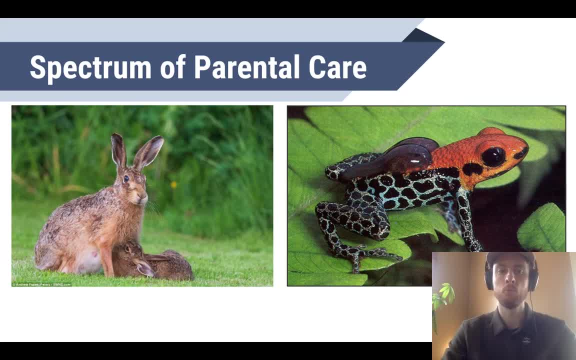 kind of parental care that a chimpanzee mother does, having one baby chimp every five years. but they're also not going to just leave their numerous offspring to fend for themselves like the oyster. So now we're going to talk about invasiveness and we're going to talk about 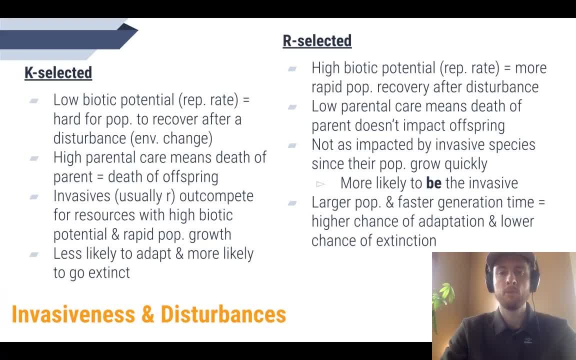 disturbance. So, like I've said earlier, both of these reproductive strategies work to pass on their genes, or we wouldn't see so many organisms in both groups. But they do have some disadvantages. So the slow reproductive rate or biotic potential of K-selected species makes them slower to. 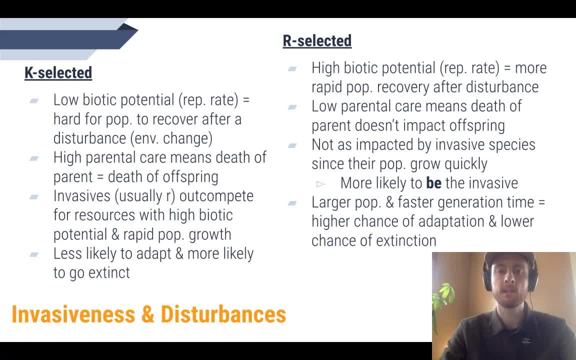 repopulate after environmental change or disturbance such as a forest fire or a disease, And then unfortunately there's kind of a double whammy effect on population recovery for the K-selected species. So we're going to talk about invasiveness and we're going to talk about 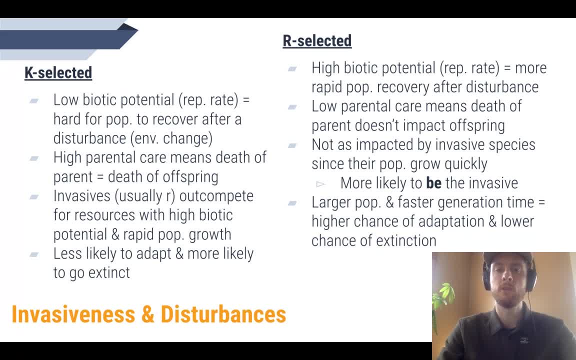 the slow reproductive rate or biotic potential of K-selected species, Since their young are born very vulnerable and usually unable to care for themselves. the death of a parent often means the death of their offspring as well, So that's more than just the one parent dying that's impacting. 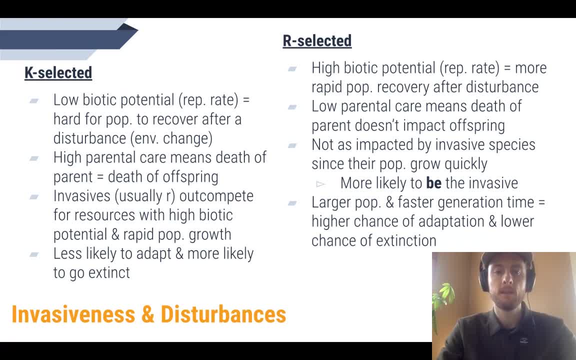 the population. It's also probably killing the offspring. Their slow sexual maturity and their low biotic potential also makes them more vulnerable to being out-competed for limiting resources by highly competitive, rapidly reproducing invasive species. So, as you may guess, these invasives are usually R-specific.